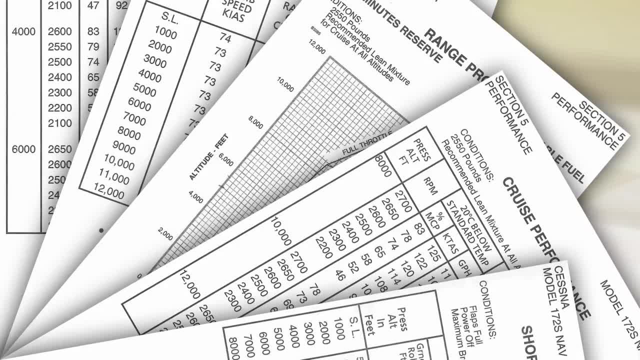 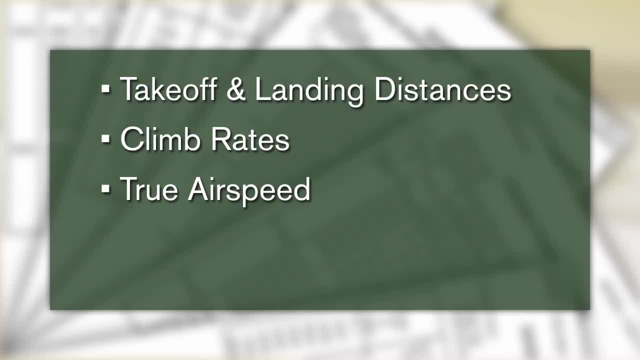 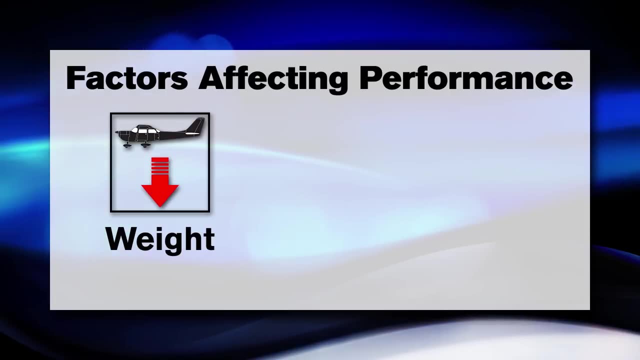 Aircraft manufacturers publish performance charts to allow pilots to calculate the aircraft's performance numbers, including things such as takeoff and landing distances, climb rates, true airspeed and fuel consumption. The two major factors that affect an aircraft's performance are… the weight of the airplane and the density of the air the airplane is flying through. 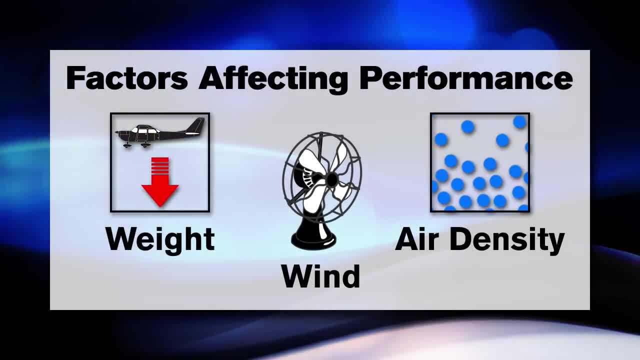 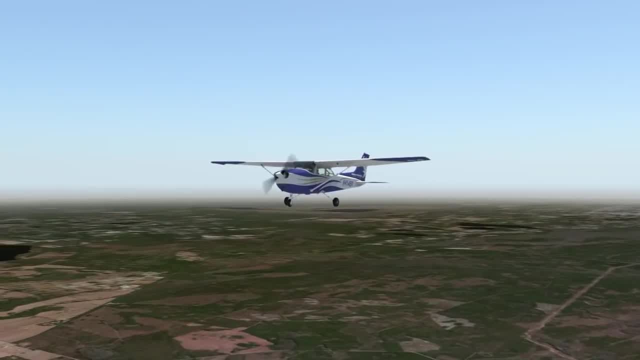 Additionally, the wind can play a factor, especially in the most critical phases of flight – takeoff and landing. We'll first look at how weight affects aircraft performance. If we consider an airplane in level flight, the wings are producing the same amount of. lift as the weight of the airplane. If the plane weighs more, the amount of lift the wings have to produce increases as well. The product of lift is drag. so if the amount of lift is increased, the amount of drag will also increase. 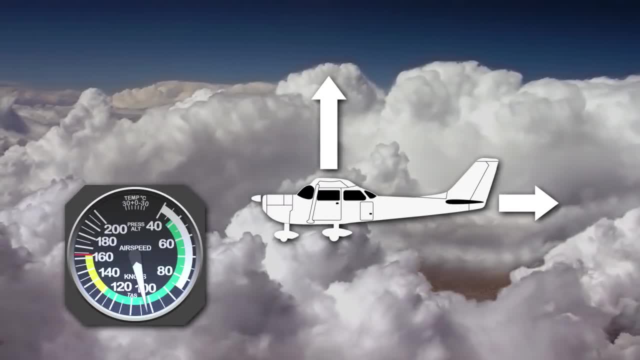 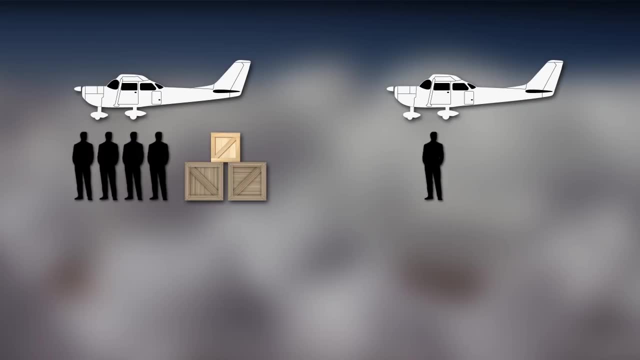 The increased drag will result in a slower airspeed for a given power setting, thus decreasing the cruise performance of the airplane. So if we load our airplane to its maximum gross weight, we will get a slower cruise speed than if we were flying at a lighter weight. 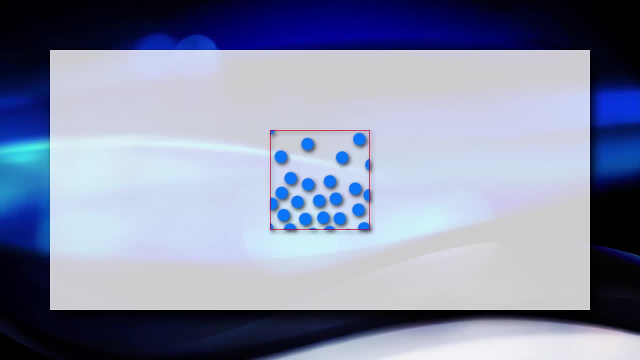 Just as important as the weight of the airplane is the density of the air. Air density is a measure of how far air molecules are flying. Air density is a measure of how far air molecules are flying. Air density is a measure of how far air molecules are flying. 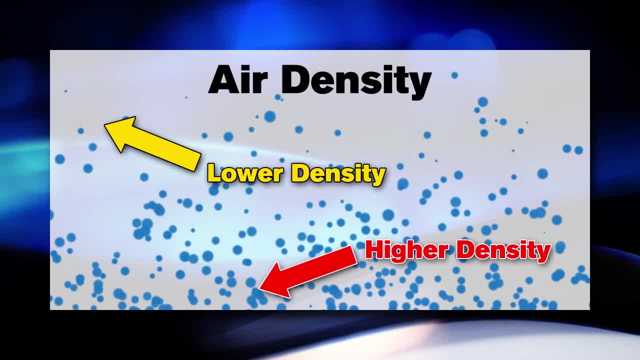 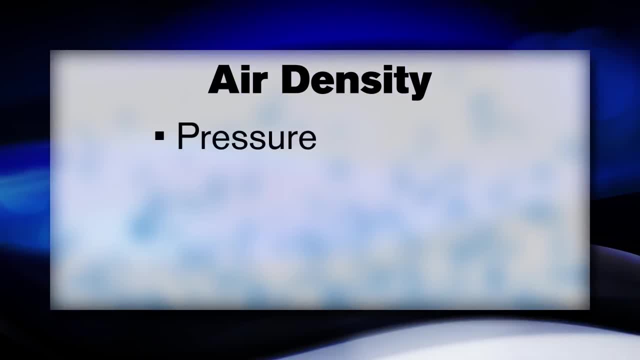 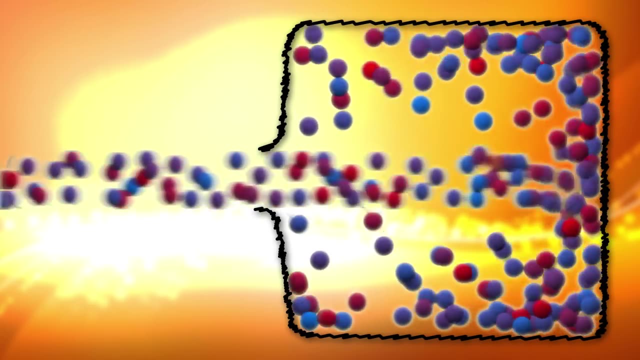 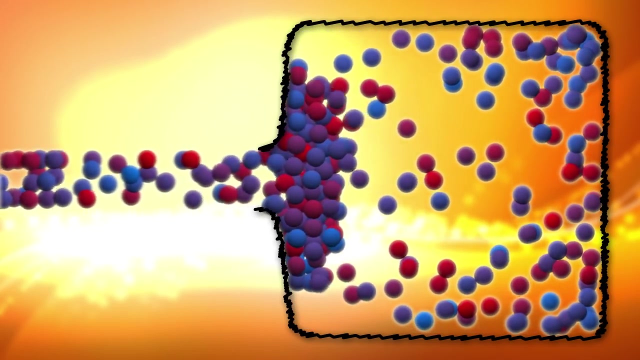 The density of the air is mainly affected by three factors, those being pressure, temperature and humidity. Pressure affects how many air particles are squeezed into a given volume of air. The less pressure applied to a parcel of air means the fewer air molecules it will contain. 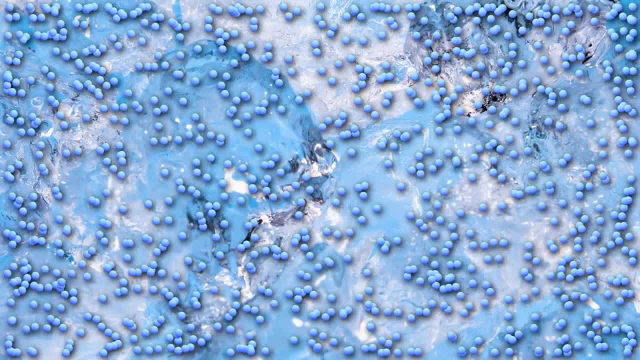 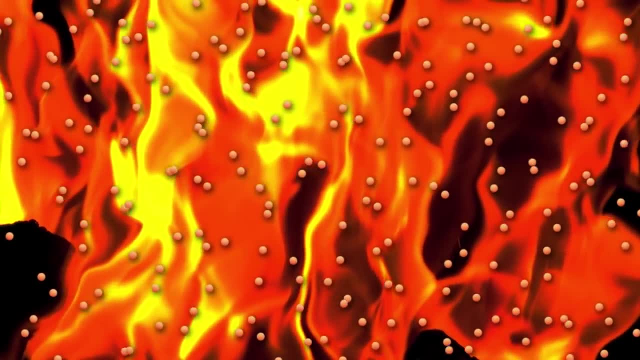 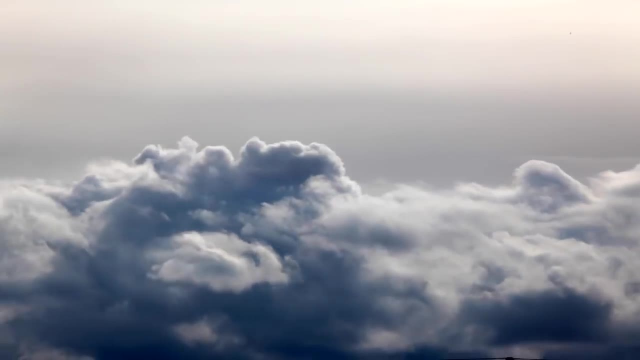 thereby resulting in a decrease in air density. Temperature also has a direct effect on air density density. The higher the temperature of the air, the more space the molecules take up as they move around. This means that higher temperatures result in a decrease in air density. One last factor to 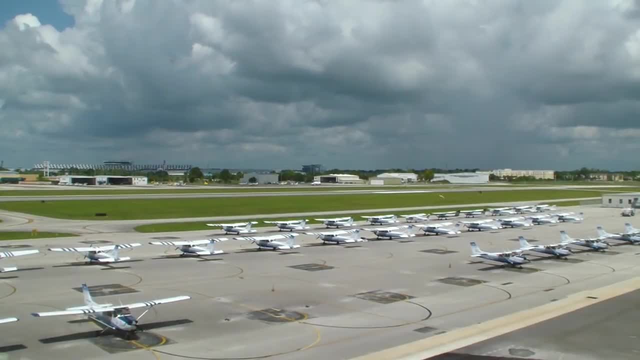 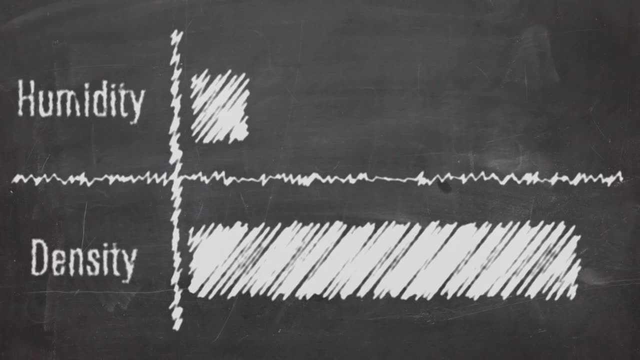 consider is humidity. Humidity alone is not considered an essential factor in calculating density, altitude and aircraft performance. However, it does contribute. The higher the humidity of the air, the less dense the air is. This is because the water vapor is lighter than 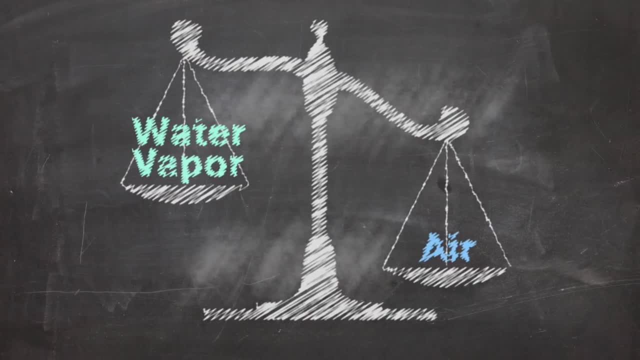 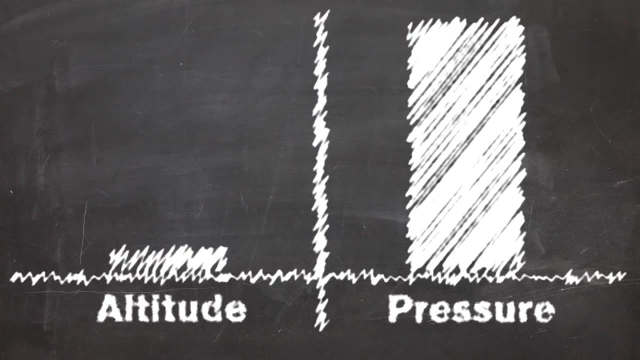 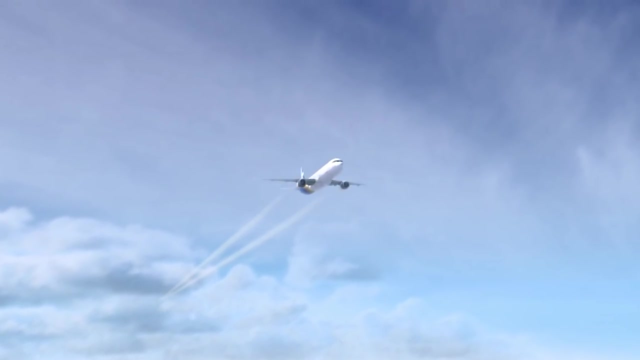 air. So the more water vapor in the air, the lower the resulting density will be. Expect a decrease in overall performance in high humidity conditions. Also, the pressure of the air goes down as altitude increases, So the higher you are flying, the lower the air pressure will be. 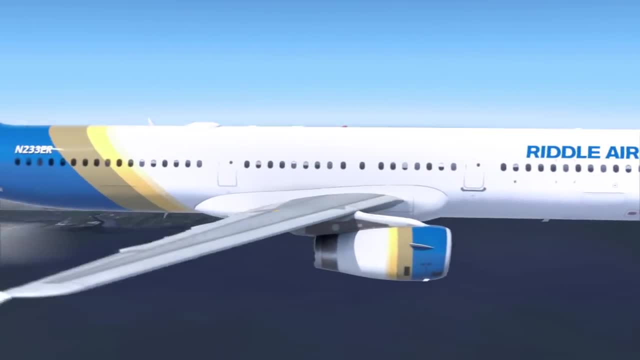 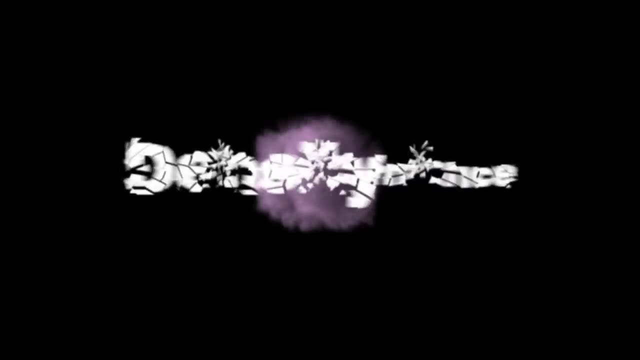 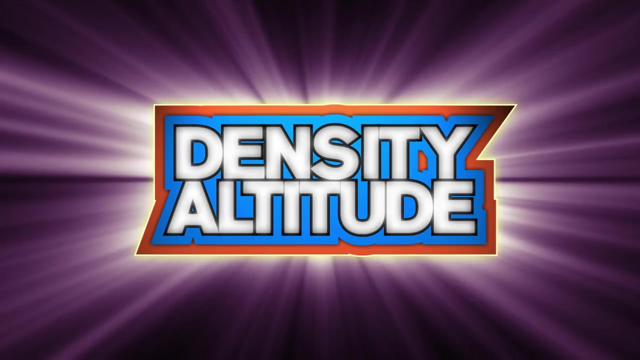 and consequently, the lower the density will be. A better way for pilots to make sense of how density affects airplane performance is to use something called density altitude. Density altitude is a way of describing how the airplane will perform when put in context of an altitude. Scientists have developed a formula that allows them to assign a specific value for 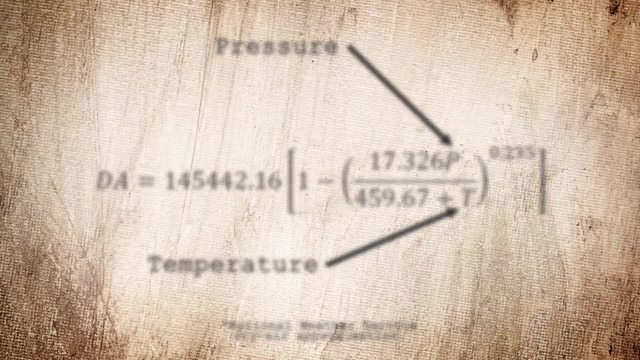 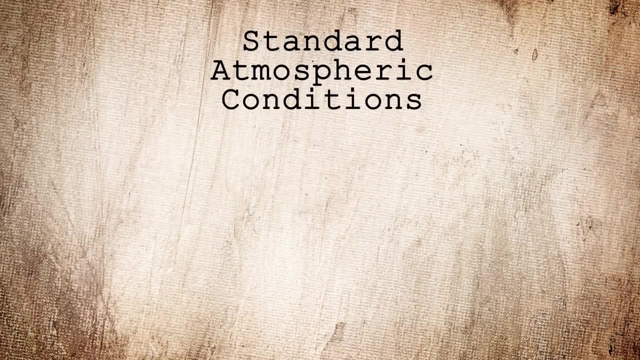 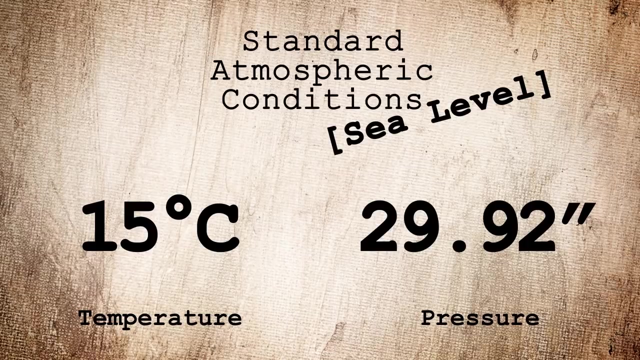 temperature and pressure to different altitudes. We call these designated values the standard atmospheric conditions for those altitudes. The standard conditions for zero feet elevation or sea level consist of a temperature of 15 degrees Celsius and a pressure of 29.5. 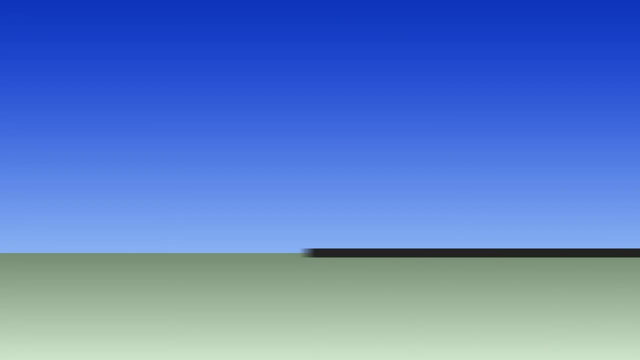 inches of mercury. Let's take an example of a Cessna departing from an airport at sea level. If the temperature is 15 degrees Celsius and the pressure is 29.92 inches of mercury, the plane would perform as if it's flying at a density altitude of zero feet. 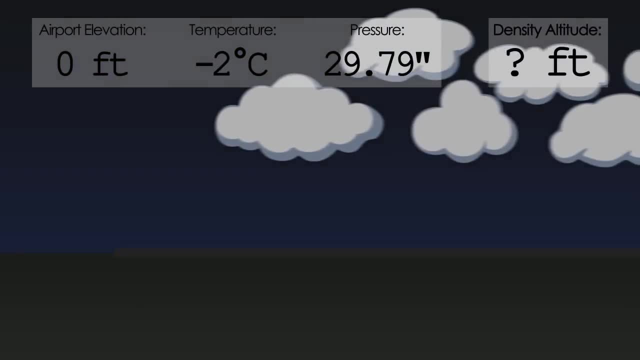 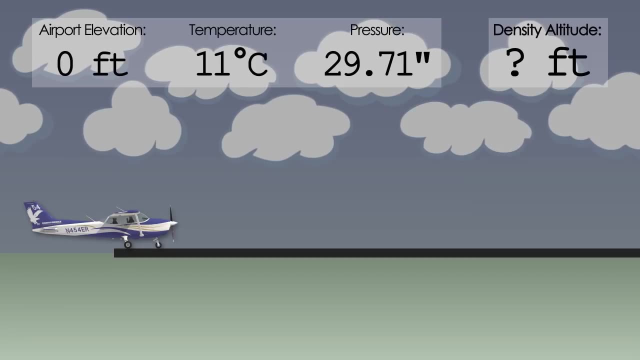 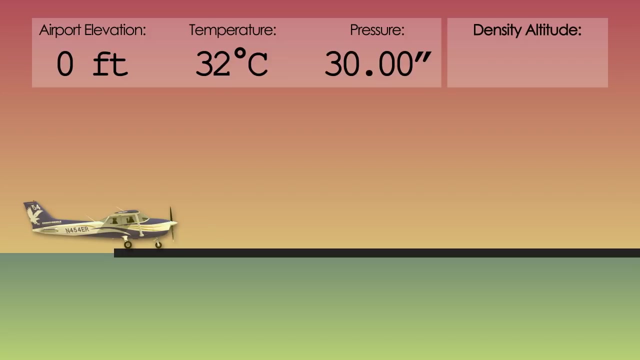 If that same airplane were to depart from the same airport on a different day with different weather conditions, we would use the non-standard temperature and pressure to determine what density altitude those conditions would represent. For instance, if the temperature was 32 degrees Celsius and the pressure was 30 inches of mercury. 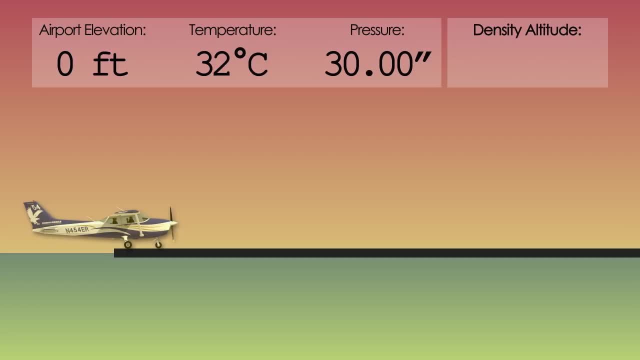 this would be the equivalent of a density altitude of approximately 2,100 feet. The pilot would then know to expect the same performance he or she would get at 2,100 feet instead of sea level. This would result in the plane using up more runway to take off. 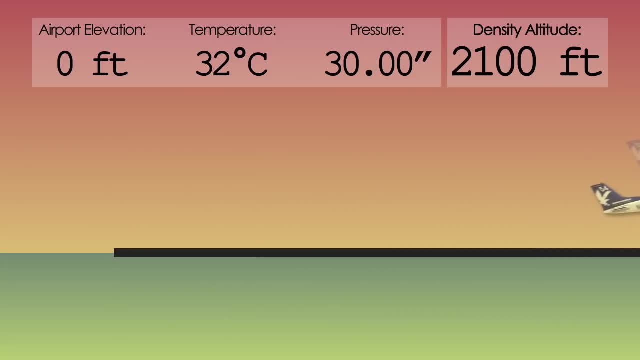 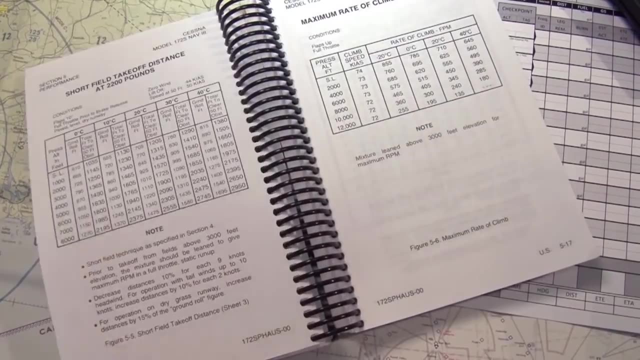 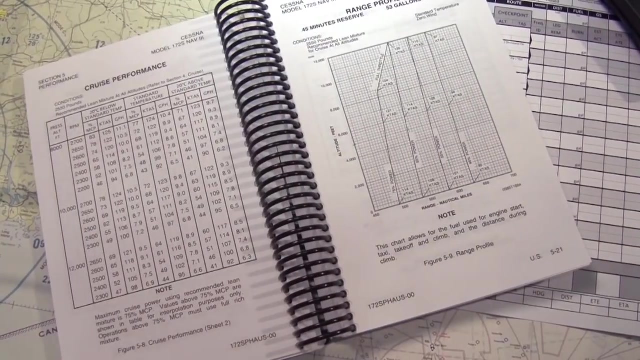 and having a slower climb up to the desired cruising altitude. Performance charts from aircraft manufacturers are published so pilots can take the changing weather conditions into account when they're calculating aircraft performance. These charts provide a simple graphical way of determining density altitude without the pilot needing to 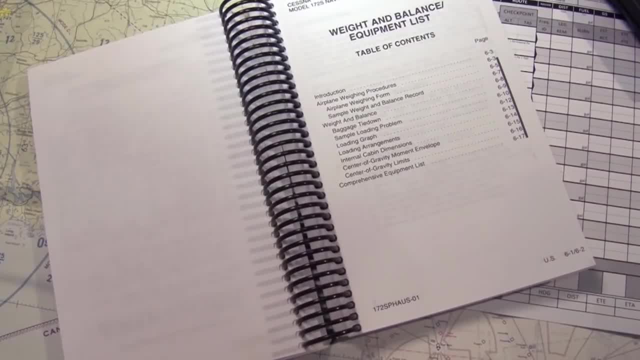 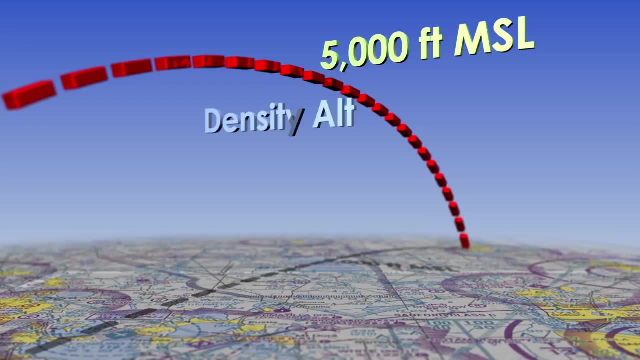 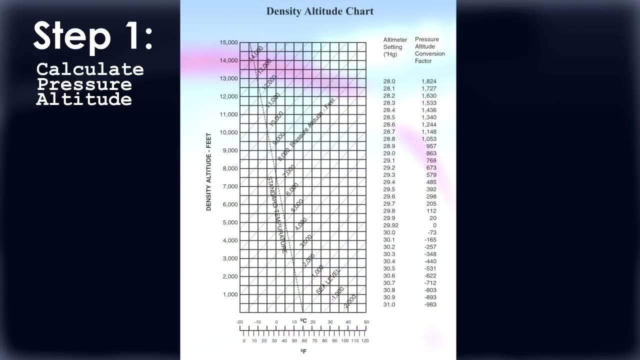 perform complex math problems to get the same results. Let's say we will be flying at 5,000 feet to our destination and want to find out what our density altitude will be. For simplicity, we'll use a density altitude chart. The first step involved is to calculate our pressure. 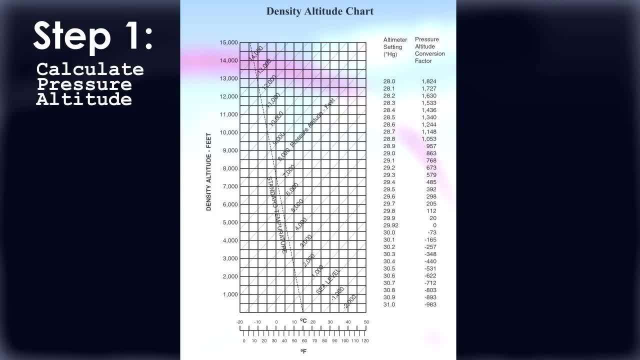 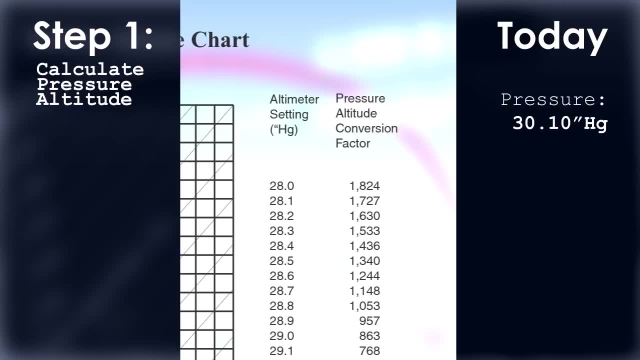 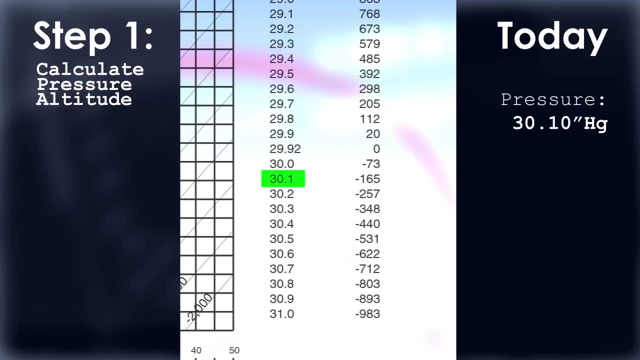 altitude which corrects for our non-standard pressure. Let's say today's pressure is 30.10 inches of mercury. Looking at the right side of the chart, we look into the left column for the altimeter setting of 30.10 and find that the pressure altitude conversion factor in the right 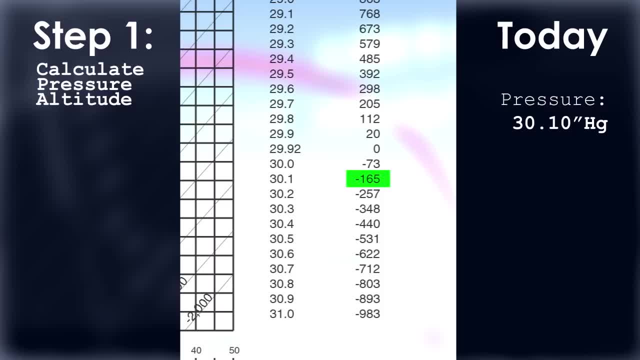 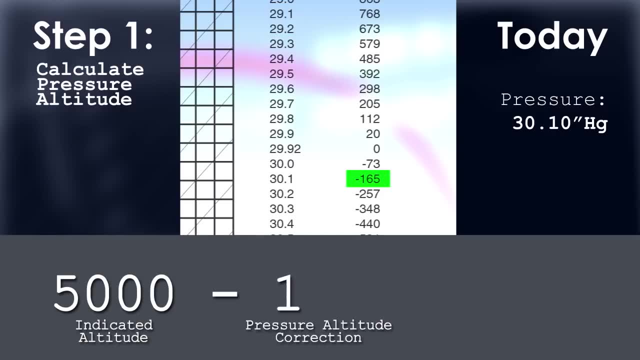 column is negative 165.. That means that our pressure altitude is one hundred and sixty-five. That means that our altimeter is one hundred and sixty-five feet lower than what's indicated. Five thousand feet minus one hundred sixty-five feet equals a pressure altitude of four thousand. 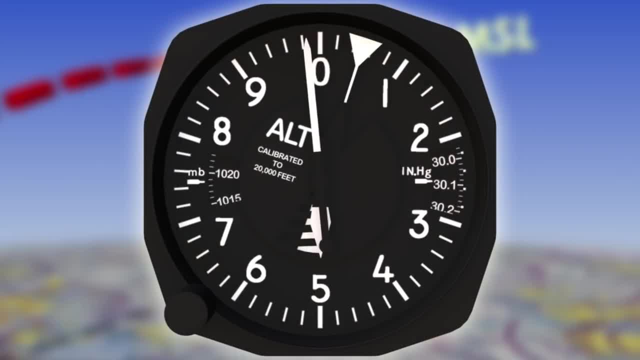 eight hundred and thirty-five feet. If we were to enter two niner point, niner two, in our altimeter's colesman window it would read four thousand eight hundred and thirty-five feet. Now that we have our pressure altitude, we need to correct for non-standard temperature. 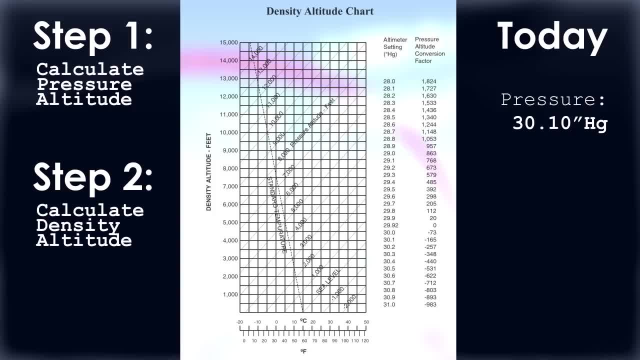 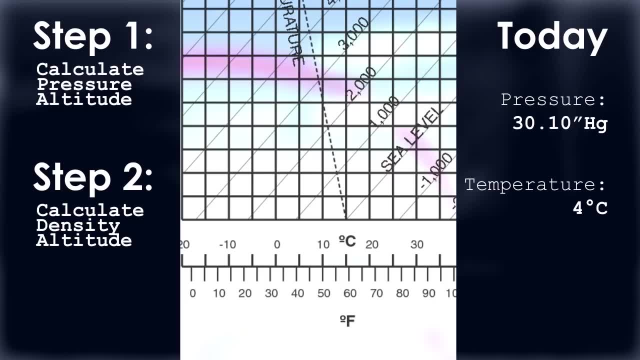 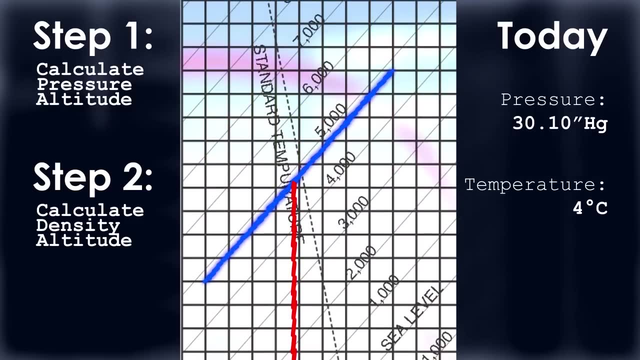 giving us our density altitude. Let's say that the current outside temperature read of the air is about four degrees Celsius. Starting at the bottom of the chart, find the four degree mark. Next follow the vertical lines upward until we intersect the diagonal pressure altitude of four thousand eight hundred and thirty-five feet. Then 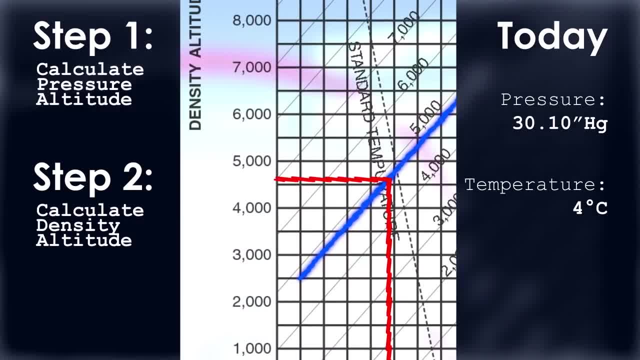 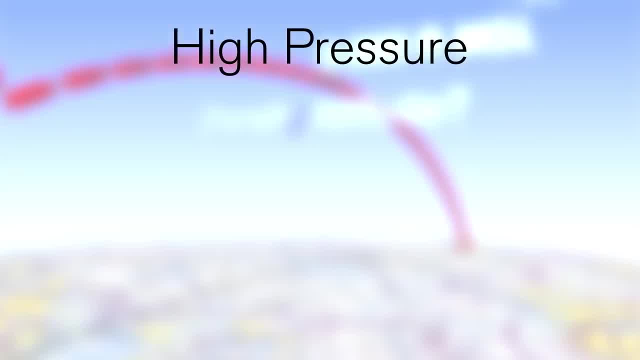 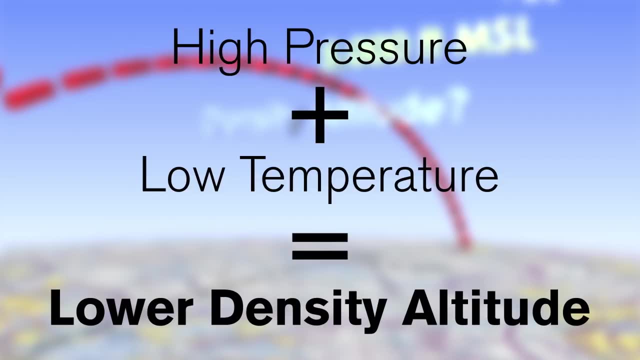 follow the horizontal lines to the left edge and read the altitude. That would result in the approximate altitude of four thousand six hundred feet. Today's relatively high pressure and low temperature resulted in a lower density altitude, Which means the plane will perform as if it were flying at a lower altitude. 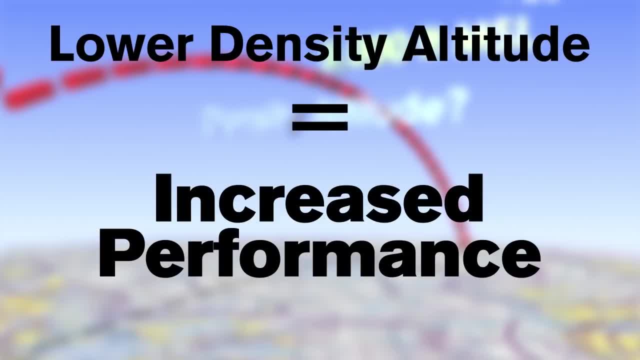 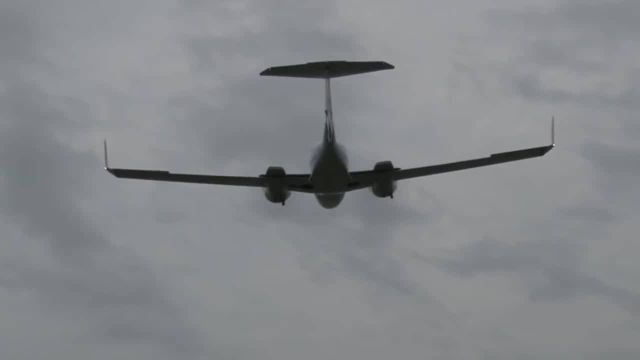 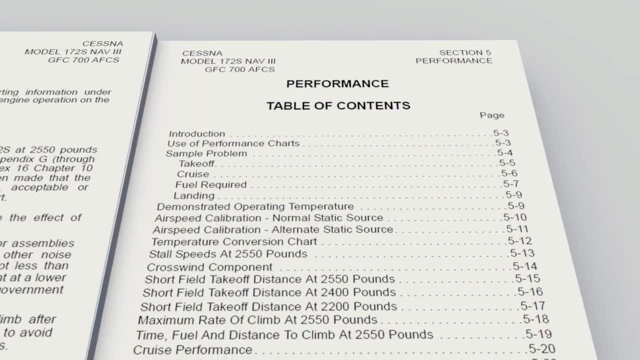 giving it an increase in performance. So now that we are able to determine pressure and density altitudes, we can take a closer look at how this affects the airplane. To see some examples of how the performance will change in different scenarios, let's look at chapter five of the Cessna 172S. 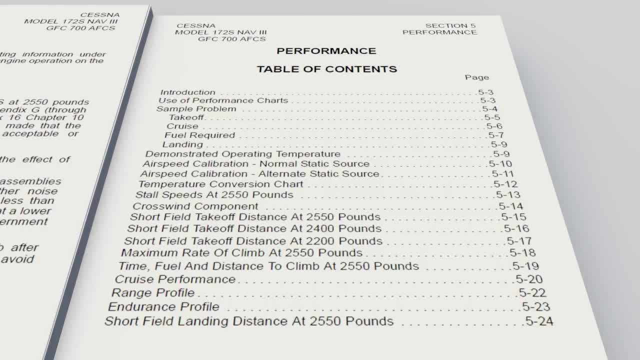 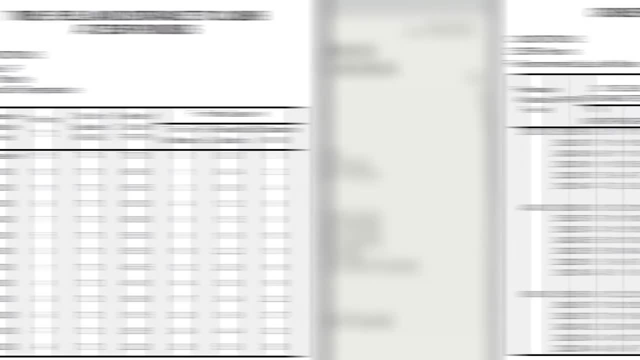 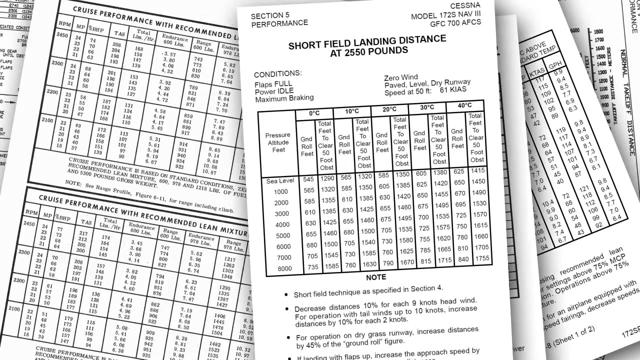 pilot's information manual. The pilot's information manual contains performance charts for the different phases of flight, including takeoff, climb, cruise and landing. Remember that each aircraft manufacturer creates their performance charts differently, so be sure to study them carefully before you actually use them. Let's start off by looking at the short. 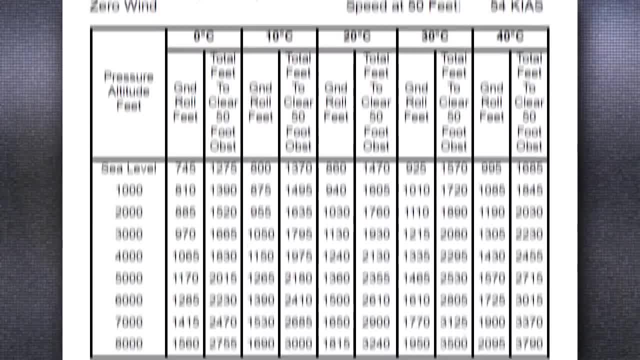 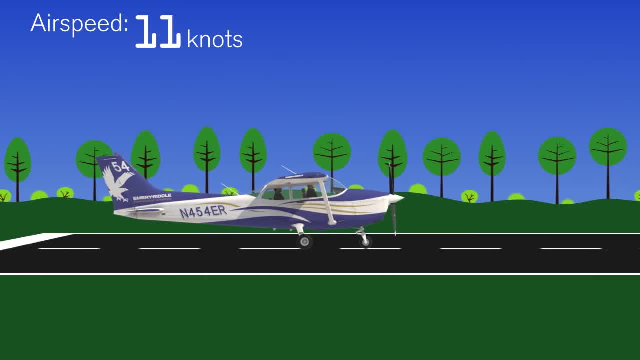 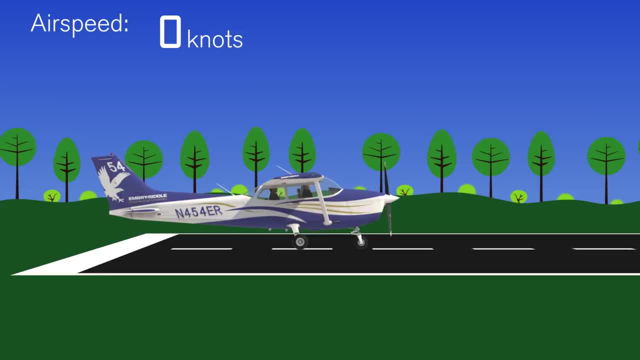 field takeoff distances for 2,400 pounds. The distances shown are for ground roll and for clearing a 50-foot obstacle. The aircraft's ground roll is how far down the runway the airplane must to accelerate from a standing start to a rotation speed of 51 knots. The column labeled total feet. 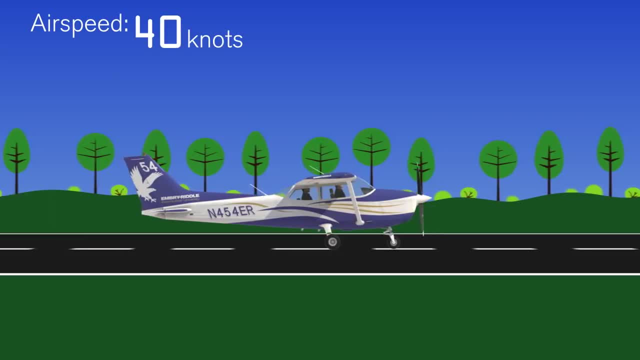 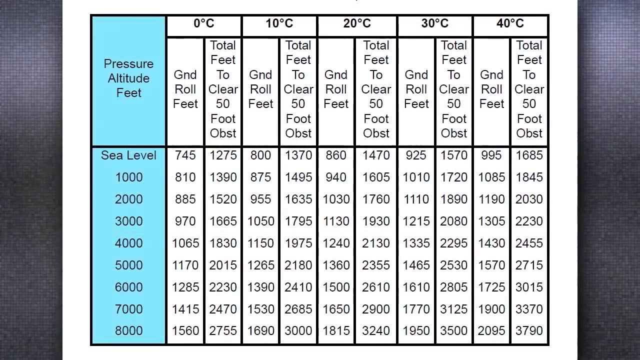 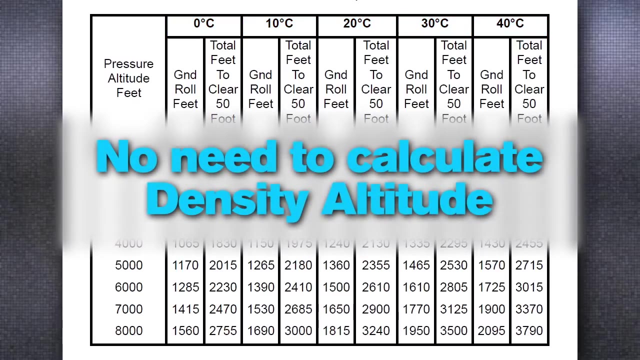 to clear a 50-foot obstacle gives the distance the plane will travel, accelerating from a standing start to takeoff and then climb to an altitude of 50 feet. On the chart, the far left column shows the pressure altitude and the top row shows temperature. In essence, the chart will calculate. 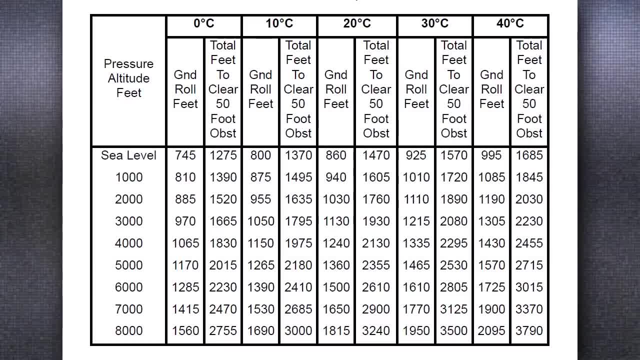 the effects of density altitude for you. Let's say, for example, our pressure altitude is sea level and the temperature is zero degrees Celsius. If we look at the intersection of these two values, we find that the takeoff distance is 745 feet As the temperature increases. 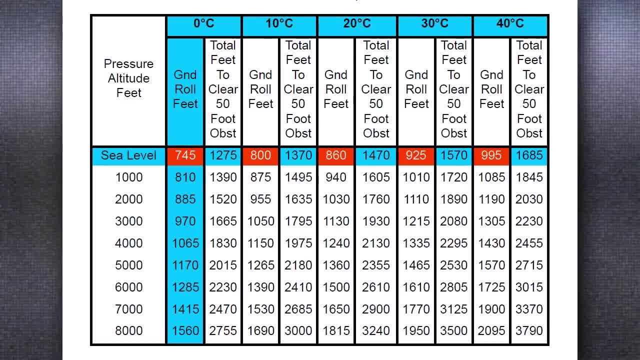 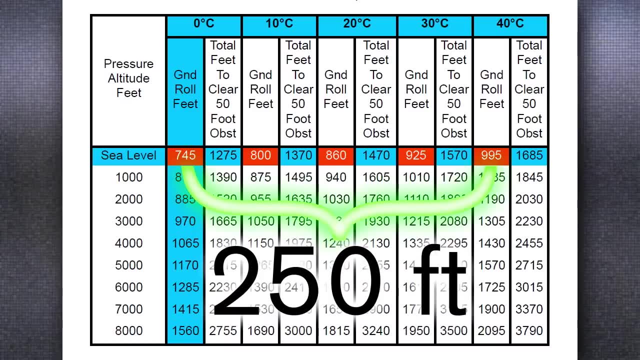 notice how the takeoff distance increases. At 20 degrees Celsius, the takeoff distance increases to 860 feet, And at 40 degrees Celsius, the takeoff distance increases to 995 feet. This results in a total difference of 250 feet increase. 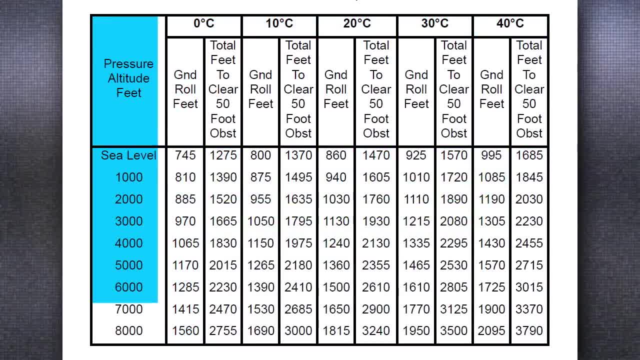 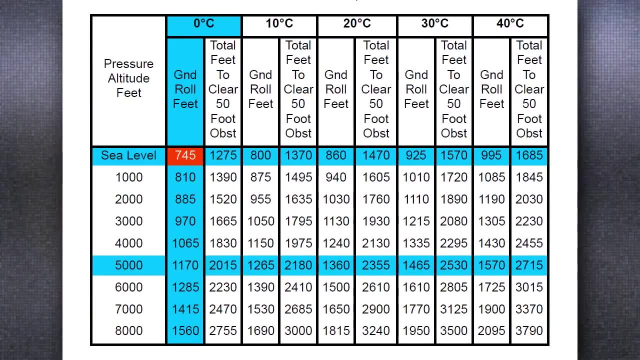 from the temperature rising. Now let's look at altitude changes. A sea level pressure altitude and a zero degree temperature results in a takeoff distance of 745 feet. At a pressure altitude of 5,000, like you would find at ERAU's Prescott Arizona campus, the takeoff roll is: 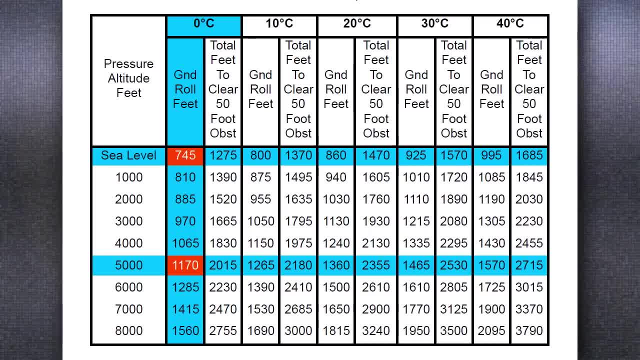 1,170 feet. That results in a difference of 425 feet. Now imagine a hot summer day with a pressure altitude of 5,000 feet and a temperature of 30 degrees Celsius. The takeoff distance in that situation would be: 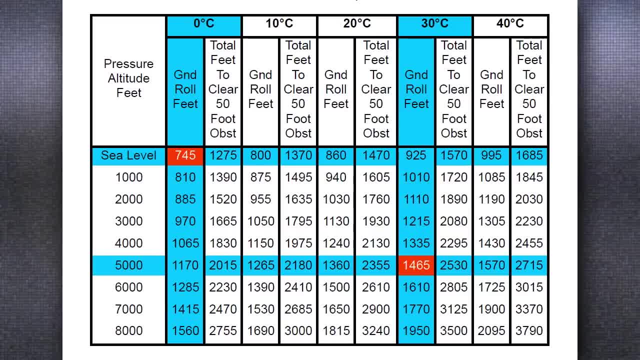 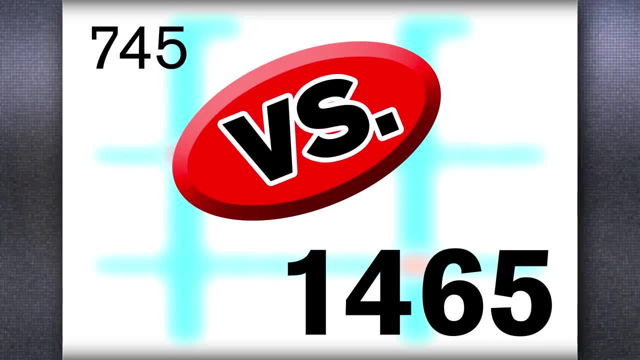 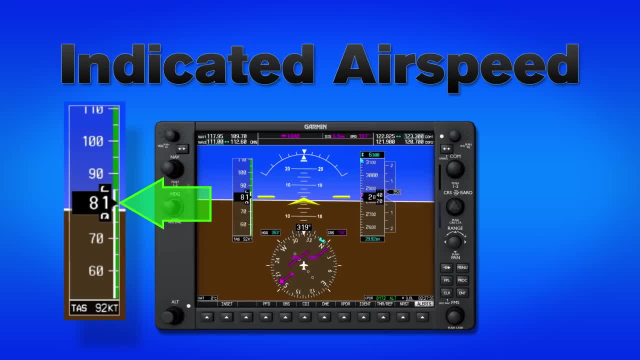 increased to 1,465 feet. That's nearly double the distance compared to what it would have been at sea level and zero degrees. The aircraft's airspeed indicator reads off what we call indicated air speed. This airspeed only takes the pressure of the air into account, instead of all of the 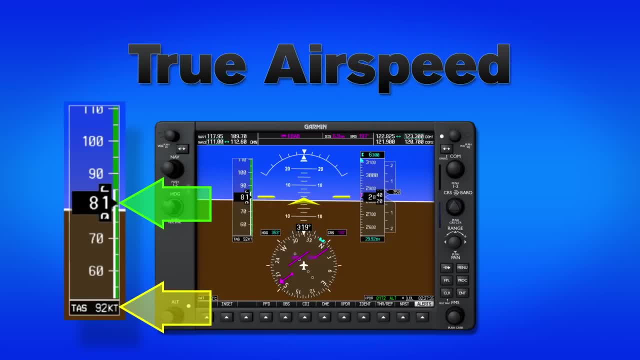 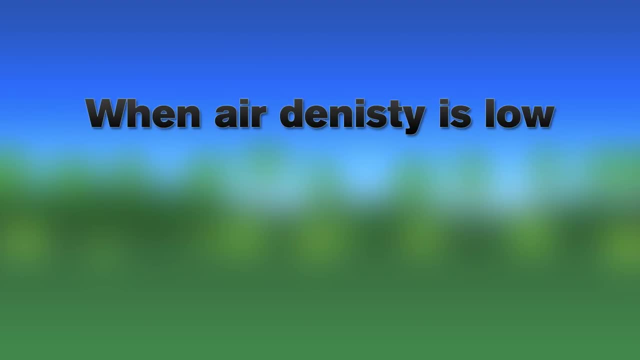 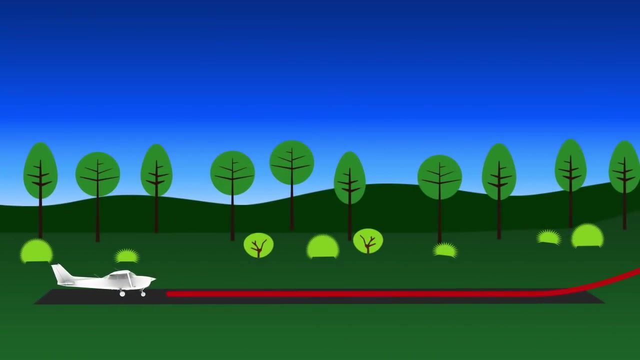 density factors. Because of that, our true airspeed be different from the indicated, depending on the temperature and humidity. On days where the air density is low, the aircraft will have to travel faster to get the same indicated airspeed. This results in increased takeoff distances. 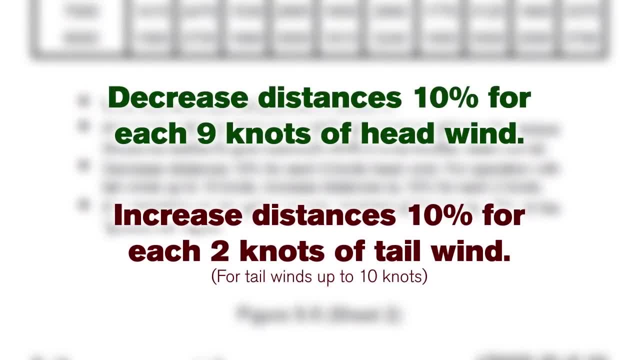 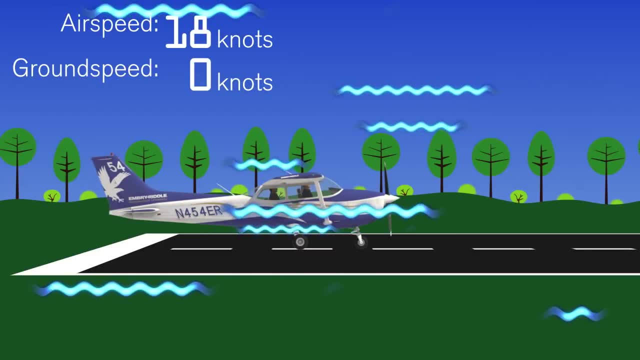 The wind direction and speed play a big role in takeoff distances as well. For the airplane to take off, it needs to reach a speed of 51 knots. If there is an 18 knot headwind, it's almost like saying the airplane has an 18 knot headstart. 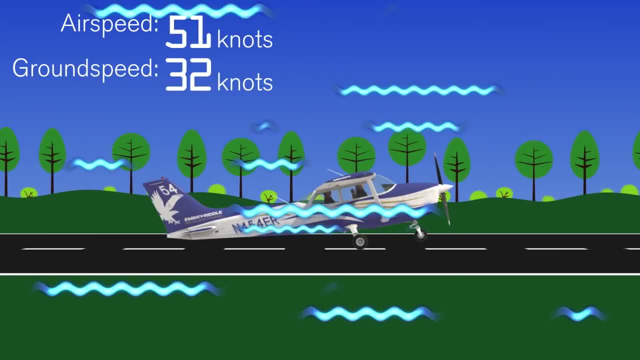 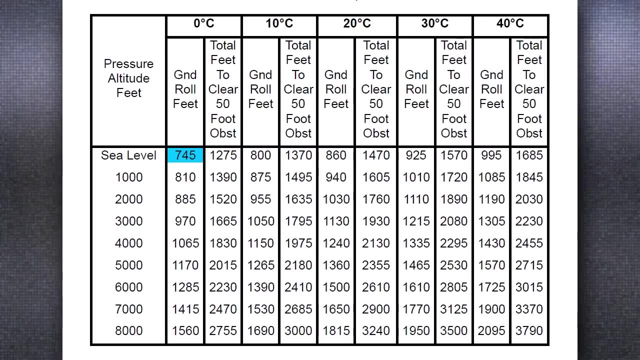 and only needs to accelerate 32 more knots to get 51 knots of wind flowing over the wings. This would reduce the runway required from 745 feet down to only 596 feet. A tailwind would do just the opposite. If we were to have a mere 4 knot tailwind, the airplane would first have to travel at 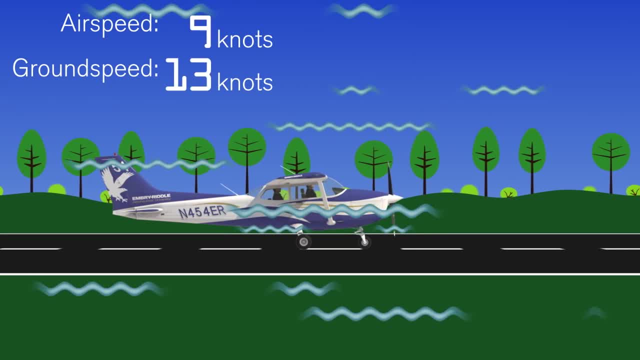 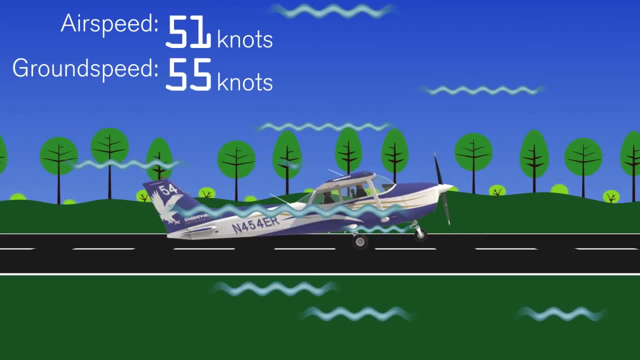 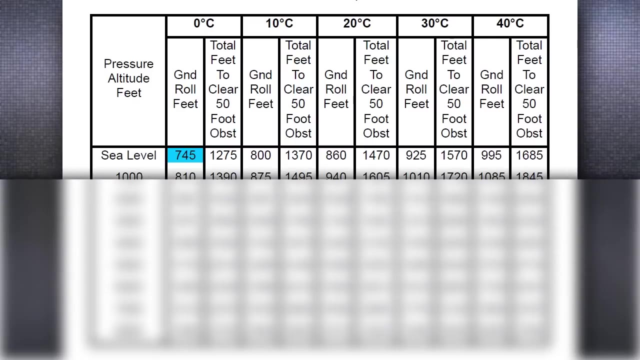 4 knots just to counteract it. It would then have to continue accelerating an additional 51 knots to be able to take off. That means that over the ground the plane would have to accelerate up to 55 knots to take off, And while a 4 knot increase doesn't sound like much, that little bit of wind would increase. 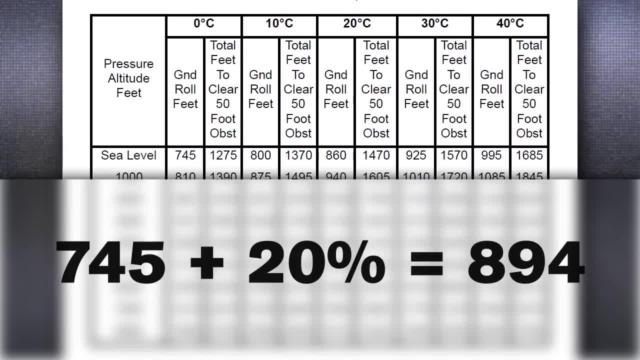 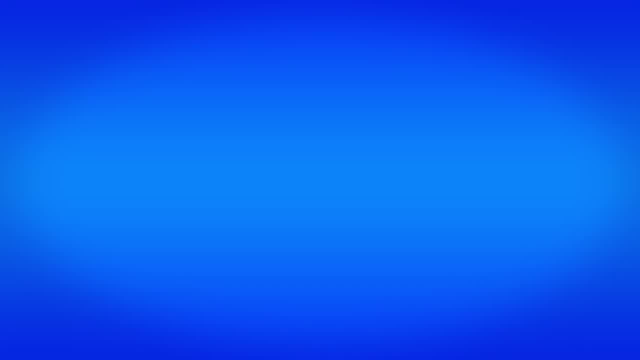 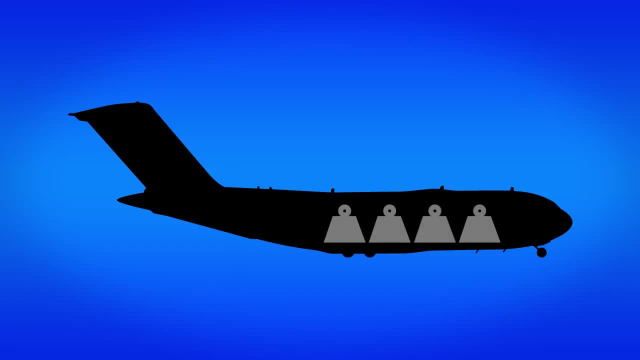 the takeoff roll to 894 feet, an increase of 150 feet. Another factor to consider in the performance of an airplane is its weight. Heavier airplanes require more power and thrust. Simply put, the heavier the airplane is, the lower its performance would be. 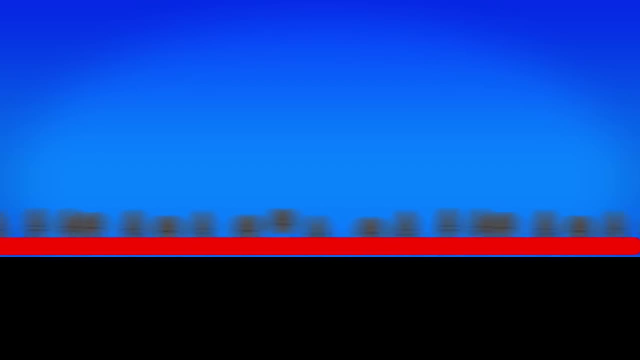 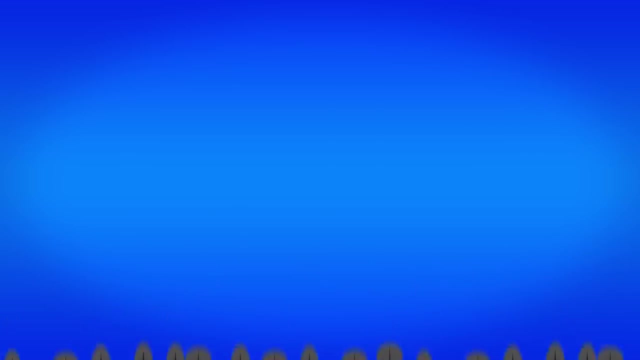 For takeoff distances. a heavier airplane would need more distance in their roll. This is because it takes more power to get the airplane rolling and accelerate to rotation speed. If we stick to our sea level pressure, altitude and zero degree temperature, the 2400 pound 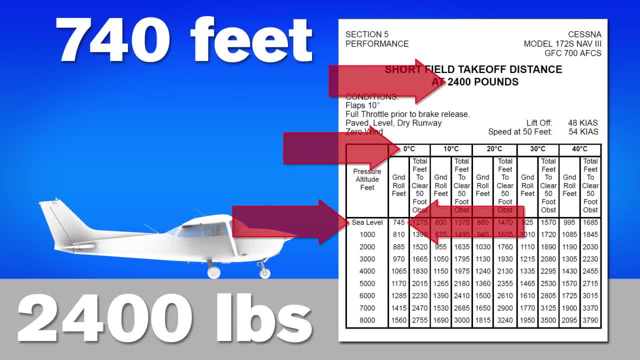 Cessna would require a takeoff distance of 745 feet. If the weight was increased to 2550 pounds, the Cessna would require a takeoff distance of 745 feet. If the weight was increased to 2550 pounds, the Cessna would require a takeoff distance. 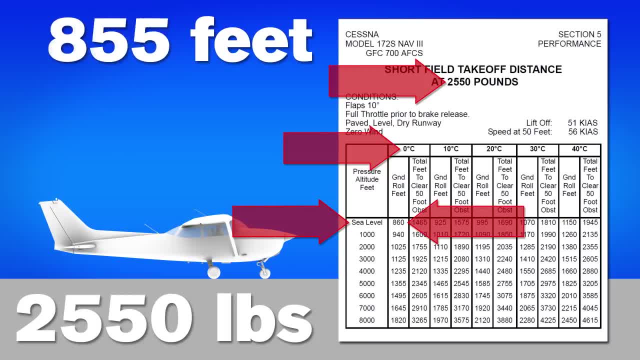 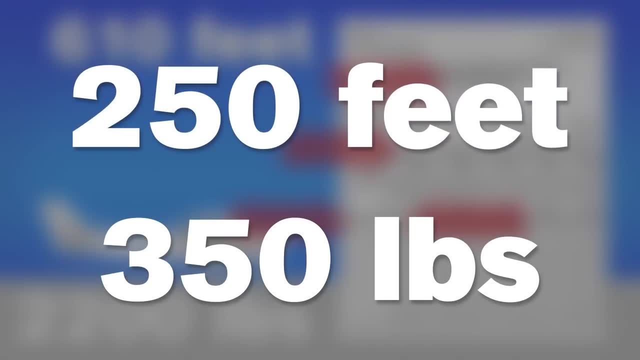 of 745 feet. If the weight was increased to 2600 pounds, the takeoff distance would increase to 860 feet. If we instead decreased our weight to 2200 pounds, the distance would decrease to only 610 feet. For those 350 pounds, we'd get a difference in takeoff distance of 250 feet. 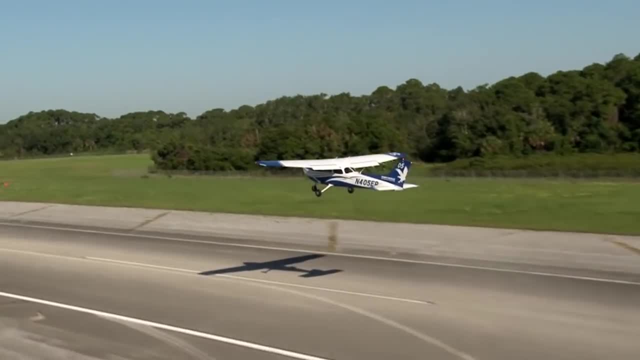 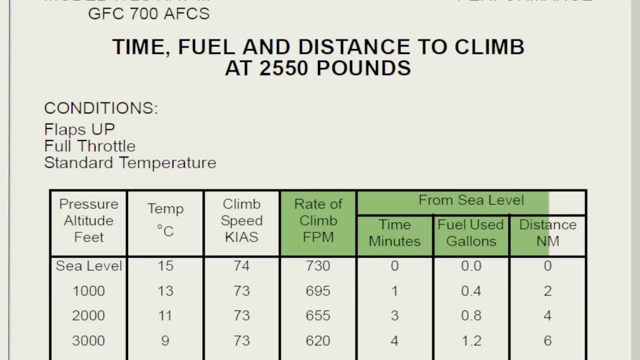 After our takeoff is accomplished, the next stage of flight is the climb. Our next chart not only shows the rate of climb that the airplane will get, but also includes the time, fuel and distance the airplane will use to get to our cruising altitude. 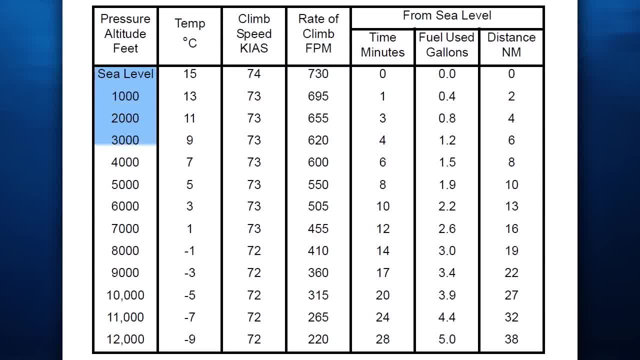 Looking at this chart, we can understand the trends as an airplane climbs higher and higher. Notice in particular how the climb rates decrease with altitude. As the airplane climbs, the density decreases and this decreases performance. So at sea level, the best rate of climb speed is 74 knots and the vertical climb rate is 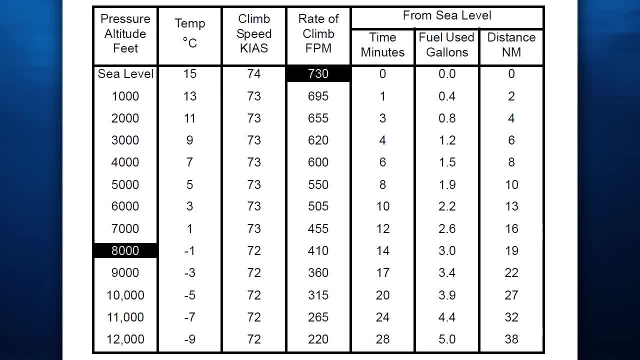 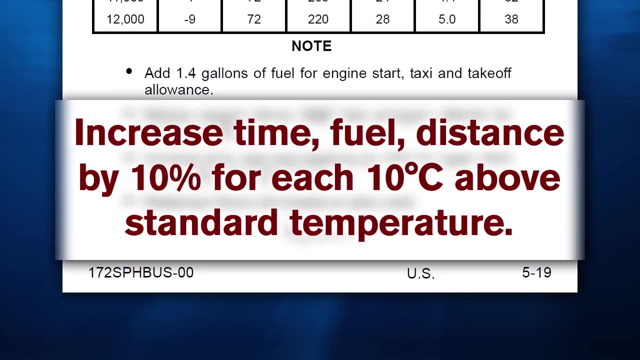 730 feet per minute. At 2000 feet the best rate speed lowers to 72, and the climb rate drops to 410 feet per minute. Temperature will also affect these numbers. The note at the bottom of the page states that all time fuel and distance numbers increase. 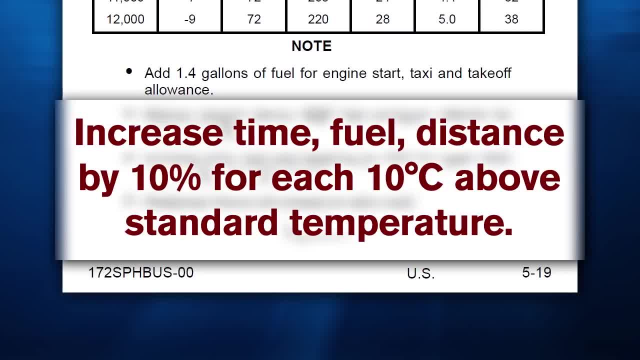 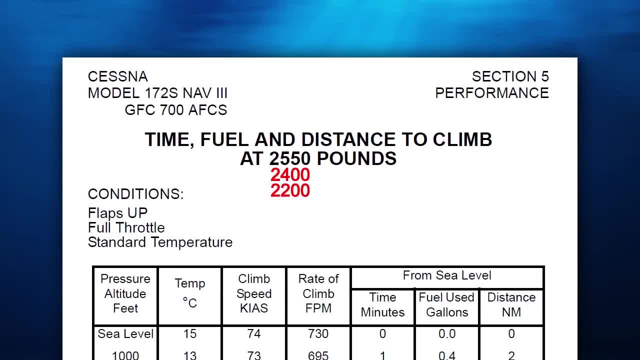 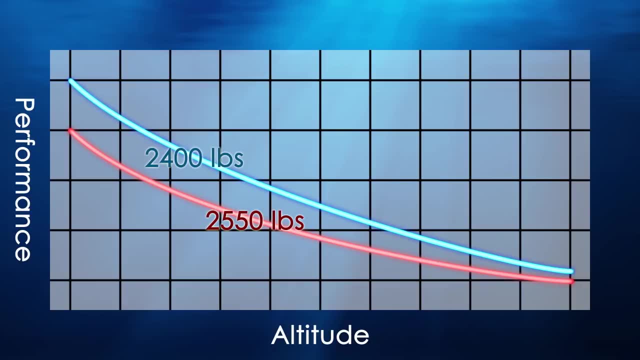 by 10% for every 10 degrees above the standard temperature. Weight changes will also affect these performance values, While Cessna does not publish the performance values at lighter weights. if the airplane did weigh less than 2,550 pounds, the airplane should climb at a greater rate than the published. 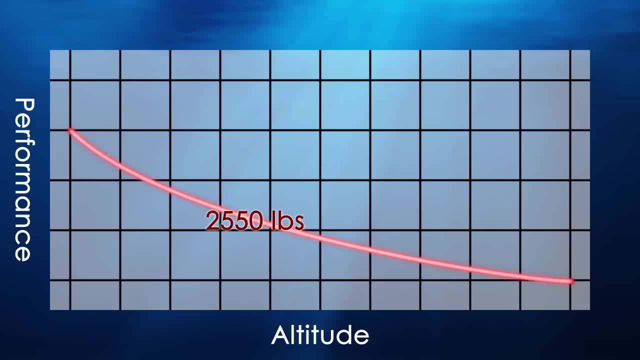 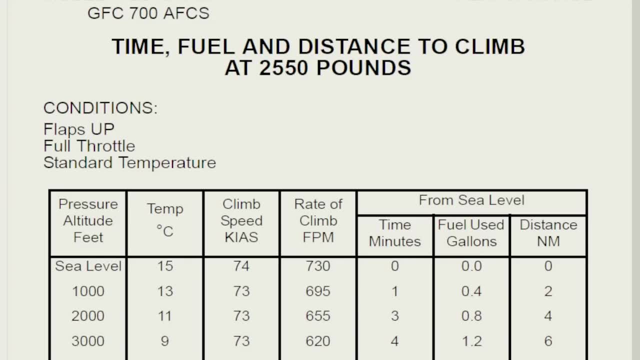 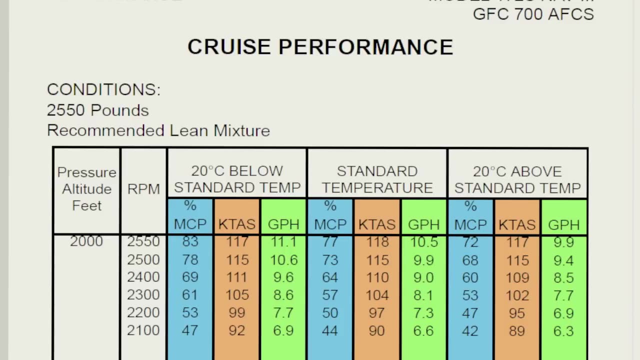 numbers. However, since Cessna does not publish the information, we plan for the most conservative scenario at the 2,550 pound weight. This next chart shows the cruise performance of the airplane, displaying the airspeed, fuel burn rate and percent of maximum continuous power in relation to different temperatures. 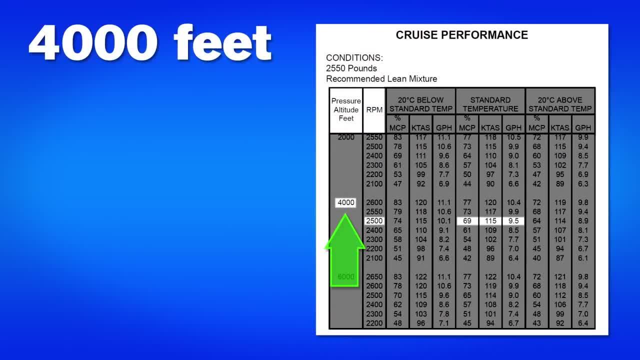 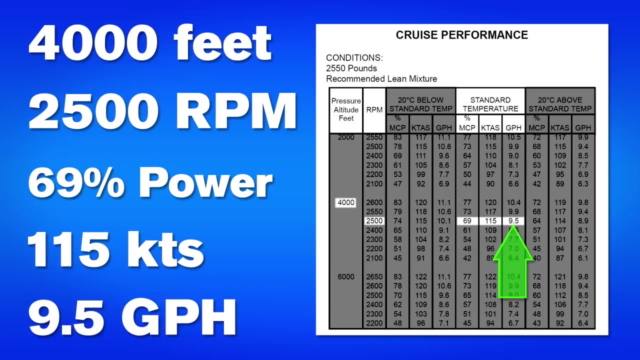 and altitudes At 4,000 feet. with an engine RPM setting of 2,500 RPM and at standard temperature, in this case 7 degrees Celsius, the airplane will be at 69% power at 115 knots and use up 9.5 gallons per hour. 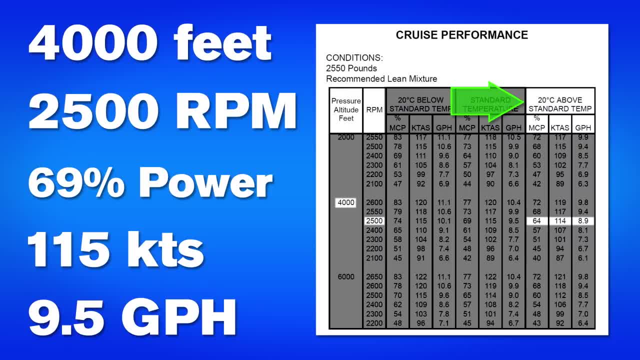 If the temperature were to rise to 27 degrees, the power output would drop to 64%, the speed would reduce to 114 knots and fuel burn would decrease to 8.9 gallons per hour. This happens without ever touching the throttle. 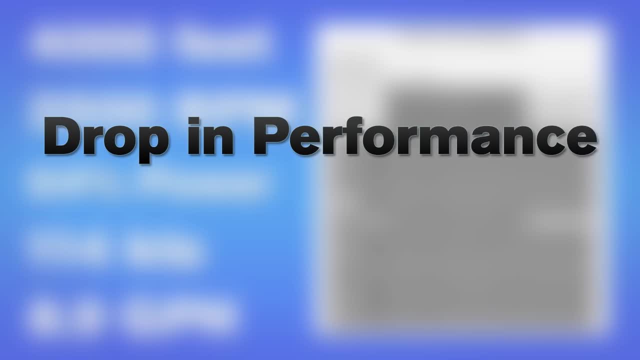 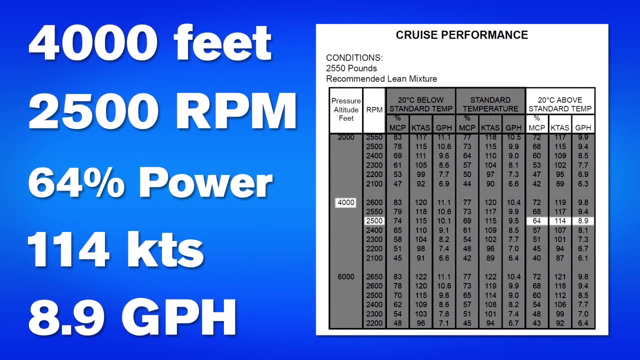 The reduced air density gives both a drop in performance and a drop in fuel burn, because the engine has less air molecules available to use. If the temperature were to drop to negative 13 degrees Celsius, the increased air density would boost the engine power to 74%, increase the speed to 115 knots and consequently, 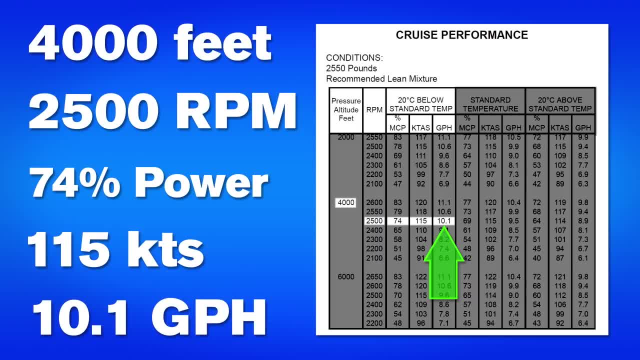 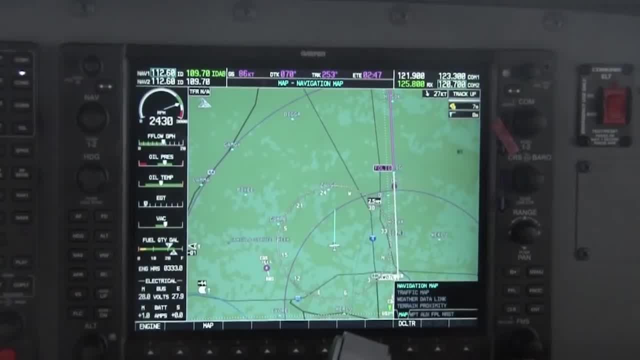 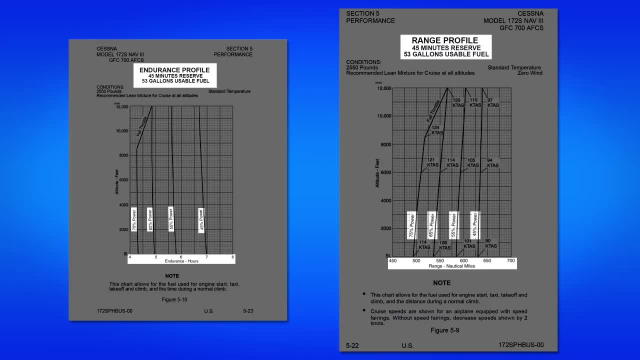 also increase the fuel burn to 10.1 gallons per hour. The different power settings available at each altitude give the pilot more flexibility in planning and choosing the one that best fits the flight plan. If we also look at the range and endurance charts, we can see how changing the RPM of 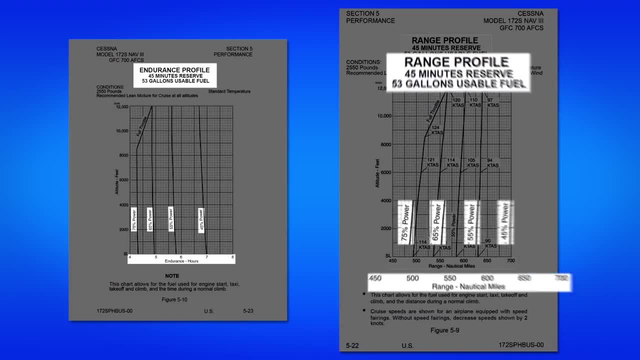 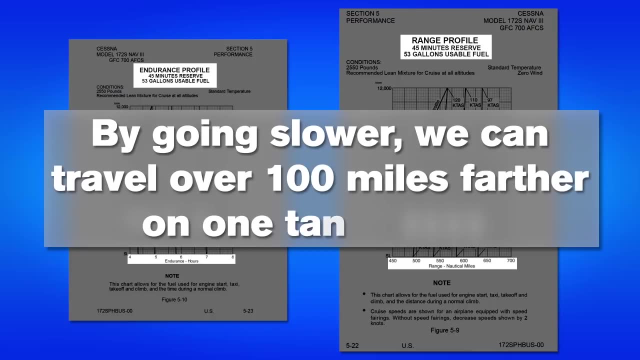 the engine can greatly affect both how far we can travel and how long we can stay in the air. By simply going slower, we can actually travel over 100 miles further on one tank of gas. If your destination is about as far away as your current maximum range, it may be wise. to slow down to a lower power setting, You'd be able to make it all the way there without needing to stop for fuel. Just like the takeoff, landing distances will also vary with the weight of the airplane, the outside air temperature and the airport field elevation. 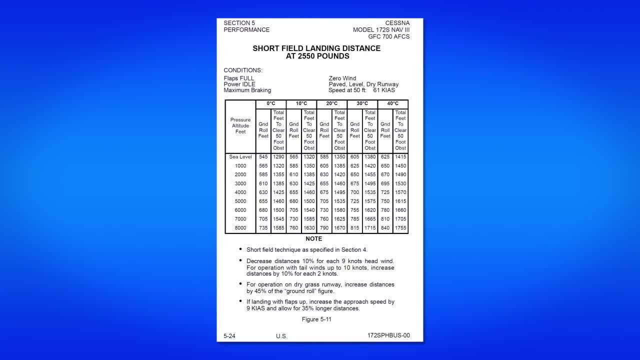 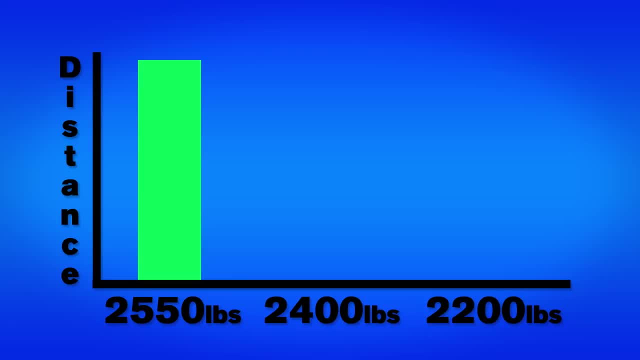 Cessna only publishes landing data for an airplane at the maximum gross weight of 2,550 pounds, but lighter airplanes will be able to fly a slower approach speed for landing and will have less momentum and less energy to dissipate once on the runway, resulting 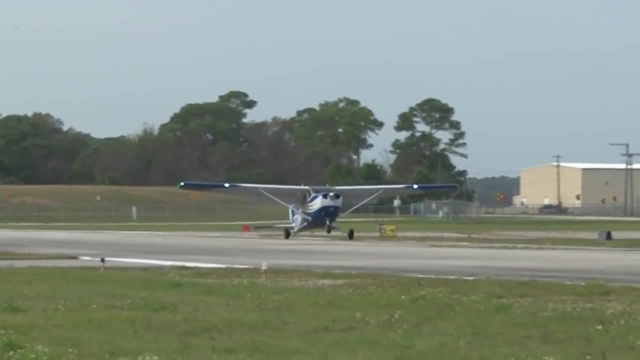 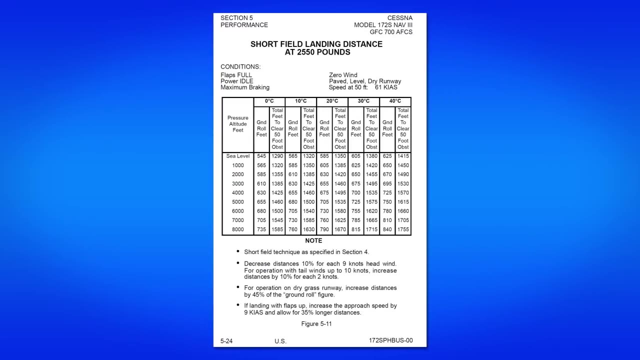 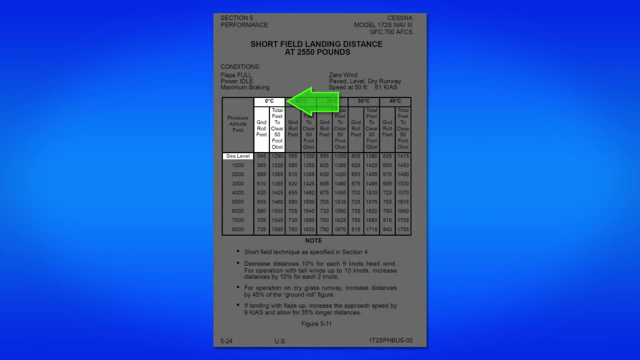 in a shorter flight time. Just like before, make sure you use the published data to calculate your runway distance required before flight. Here is how temperature and pressure affect the landing distance in the Cessna 172.. At sea level and at 0 degrees Celsius, the Cessna will need 545 feet to land. 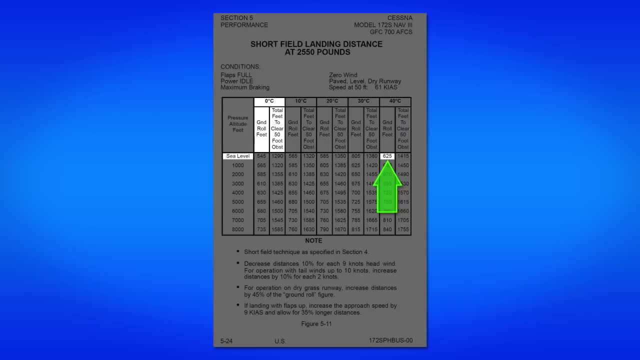 As the temperature increases, the distances increase all the way to 625 feet at the 40 degree mark. Just like the takeoff performance charts, this chart should also be taken into account. This chart shows the distance required not only for ground roll, but also for the distance. 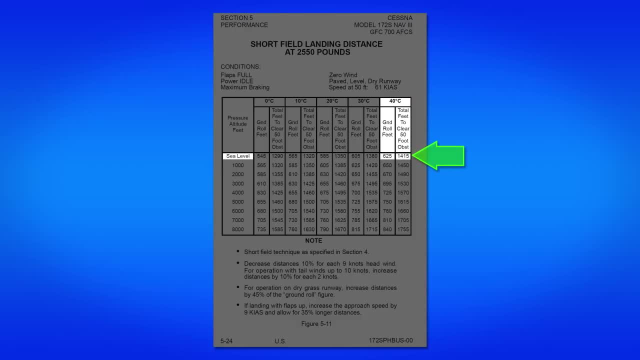 to clear a 50-foot obstacle and then land and come to a complete stop on the runway. The chart also shows the landing. distances increase as altitude increases. Here the distance of 545 feet at sea level increases to 655 feet when at 5,000 feet.